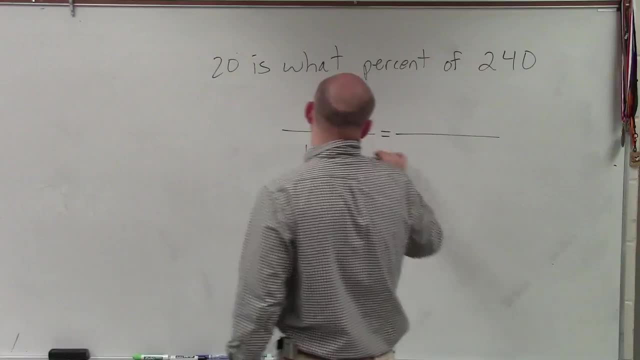 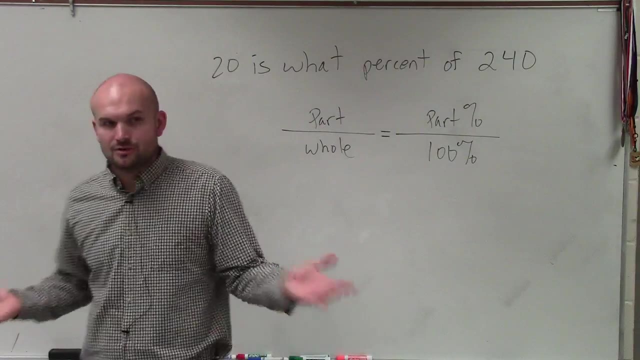 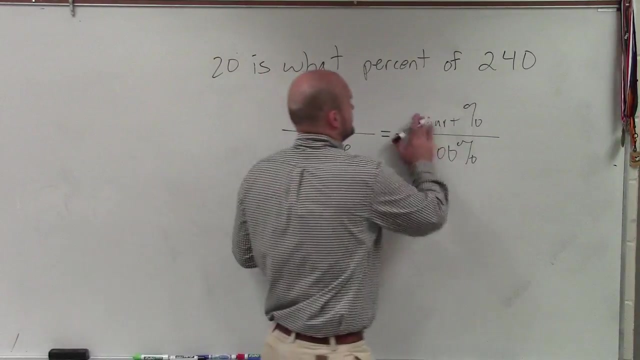 we have part over whole, part, percent over 100%. Now let's just go and figure out. do we have any percent that we have up there? No, so I have nothing to figure out for that. So that's actually what we're trying to figure out. So we'll do that as our x. Then do we have a part and a whole? 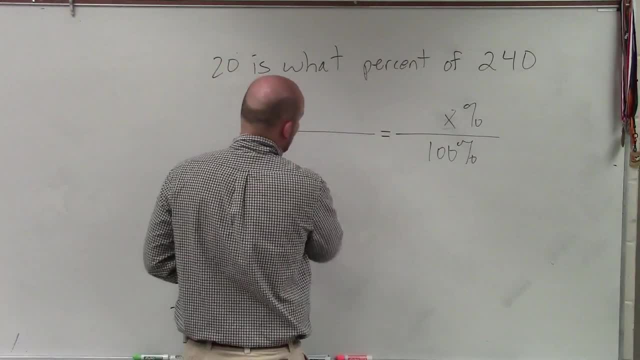 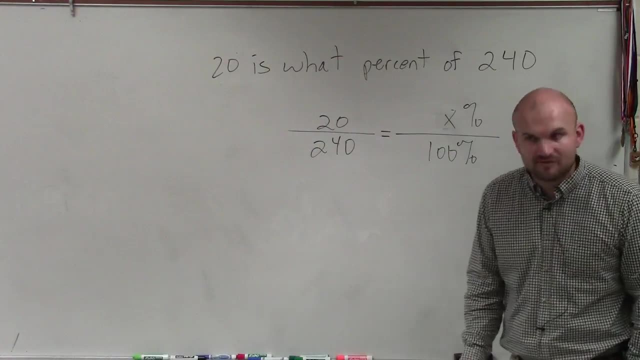 Yes, we have a part and a whole, which is 20 and 240.. Now one of the first steps we'll always want to do is simplify, simplify, simplify. right, Always simplify before we can do anything. So I already noticed I. 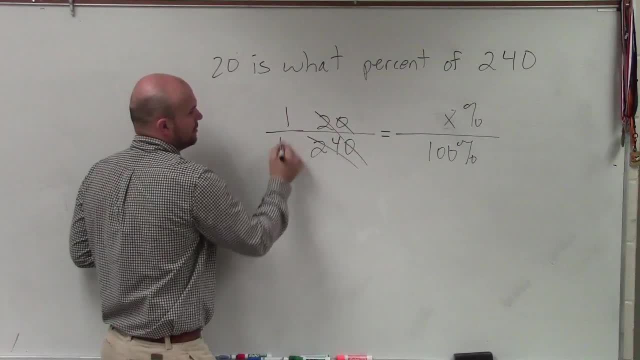 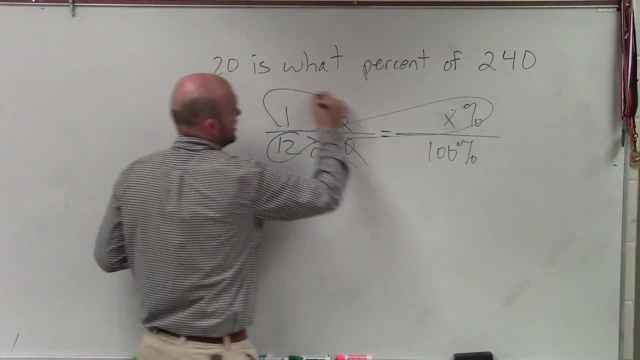 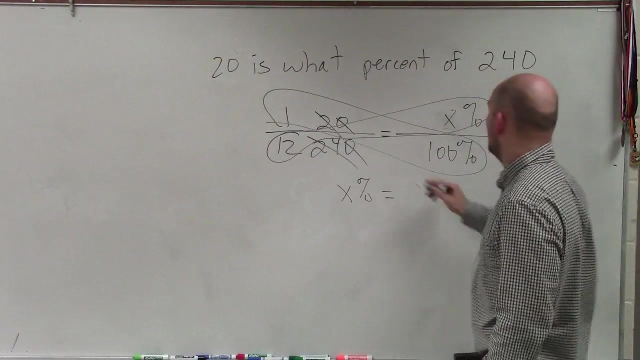 I can cancel out those zeros. I can already simplify this to 1 over 12, right, So that's not too bad. That's actually going to make this problem very simple. So now, when I apply my cross product, I have x. percent is equal to 1 times 100. 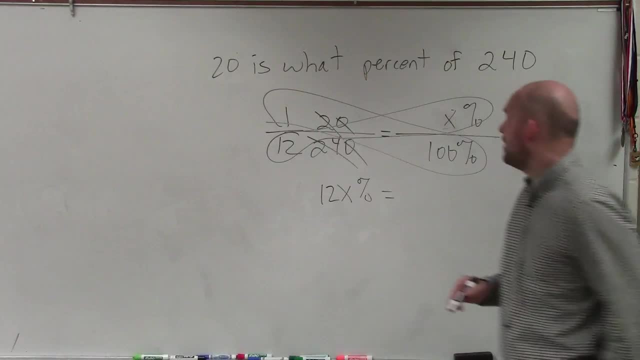 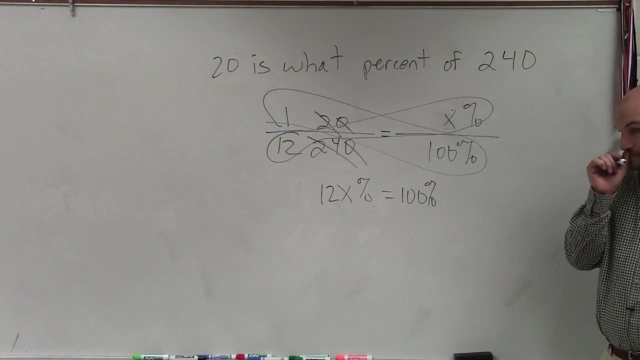 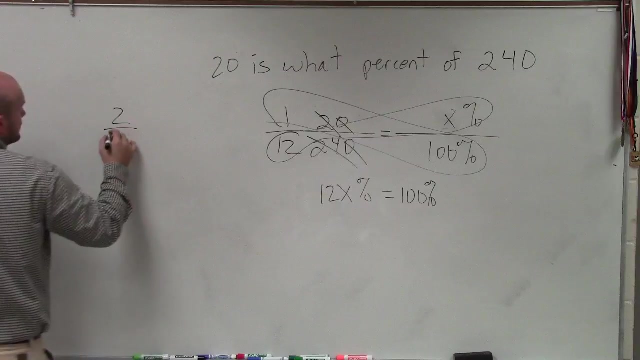 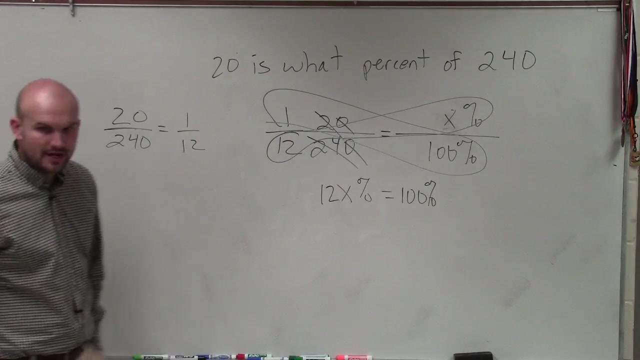 I'm sorry. 12, sorry. 12 times x, percent is equal to 100%. What here? I reduced 20 over 240 to 1, 12. That's basically me. So therefore I need to multiply 12 times the x and 1 times 100. 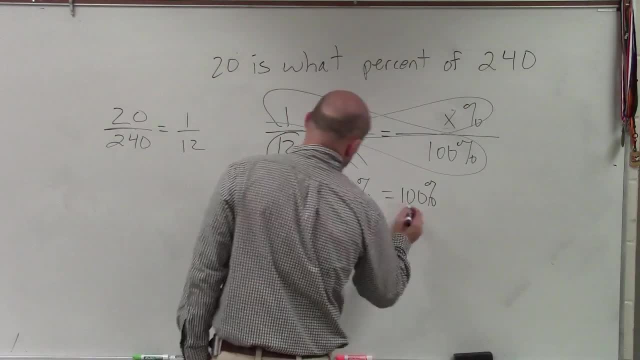 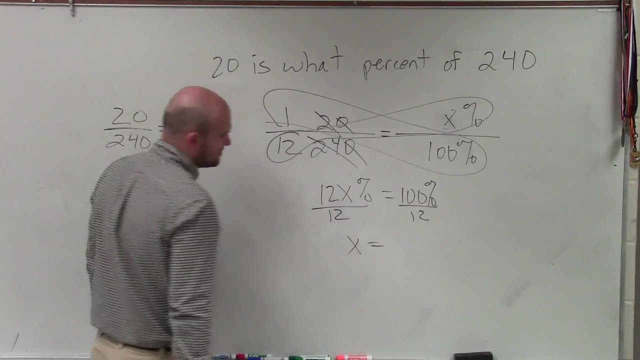 So now I just needed to divide 12 on both sides. So I'm just not going to write the x in the percent, but we can see that my answer is going to be as a percent. So now I just need to say: well, how many times? 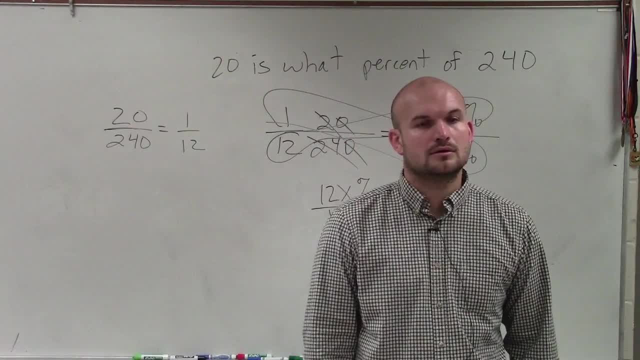 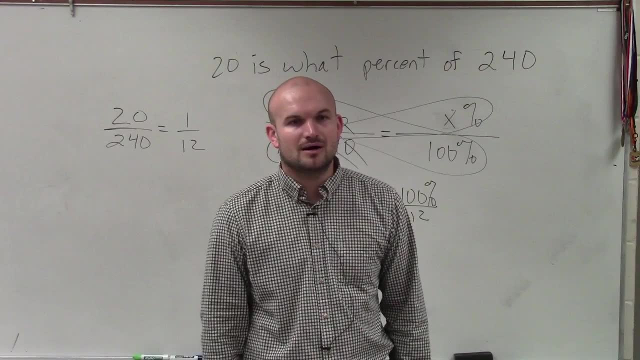 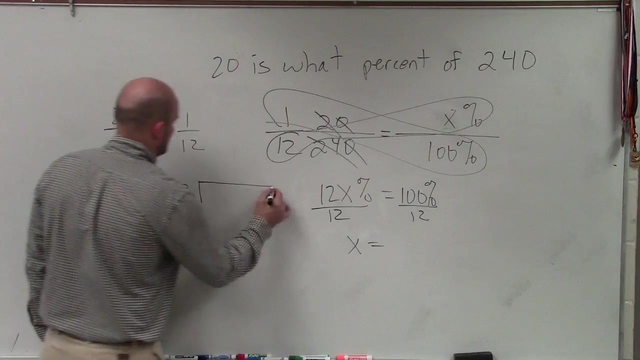 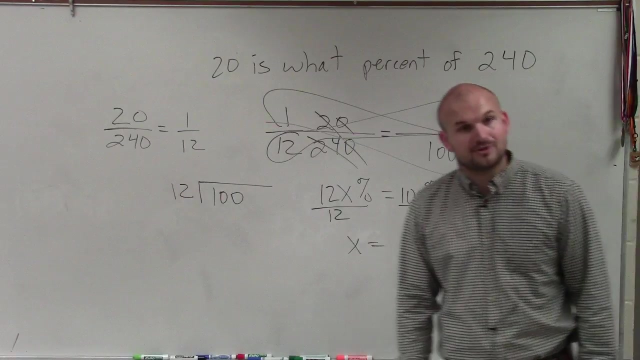 does 12 go into 100?? Still waiting for how many times x goes 12 into 100.. All right, so what we'll need to do Is go back to our handy dandy long division. all right, Because again we're doing this. 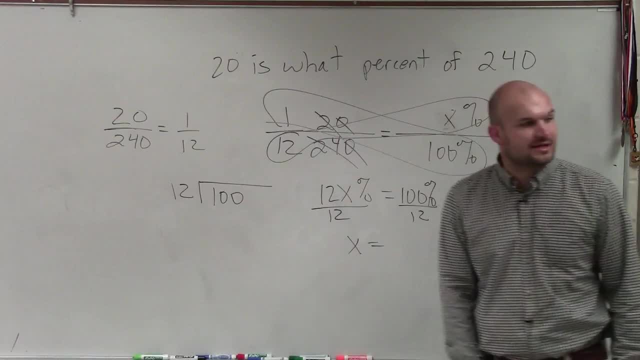 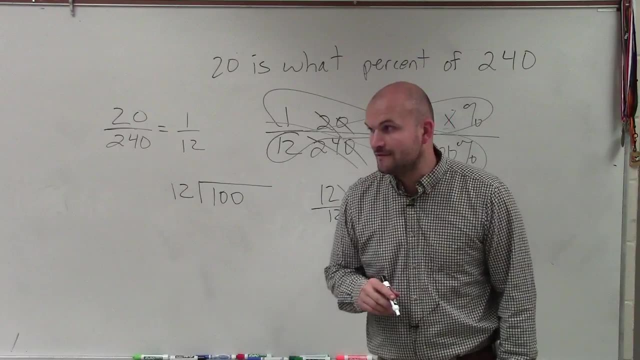 Sheldon, put your head up please. So what we're again going to do with this is again working through long division. So 12 doesn't go into 10, but 12 does go into 100.. How many times does 12 go into 100??